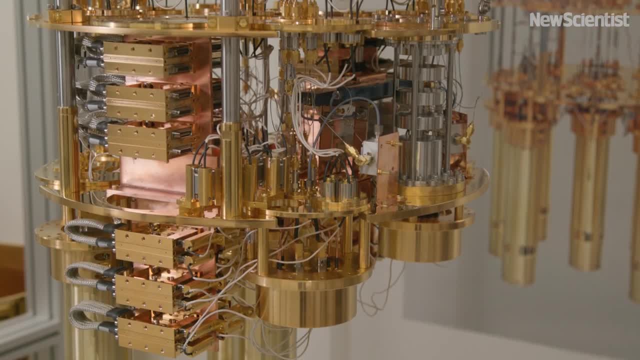 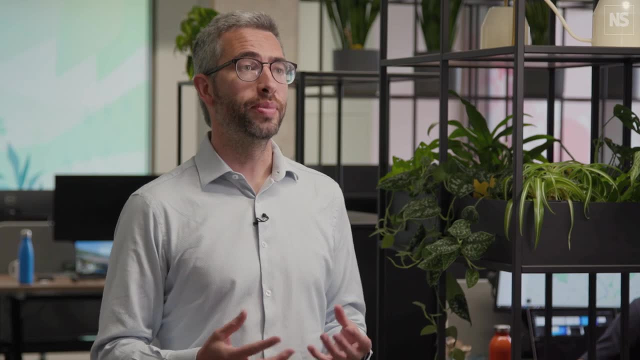 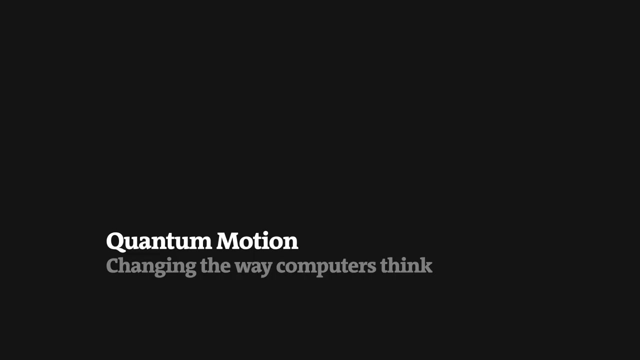 We want to build the most powerful computer on the planet, and that's a universal quantum computer. Quantum computer which is able to run any quantum algorithm. It does so by using quantum error correction and built on a platform of silicon technology, A quantum computer is the most powerful computer. 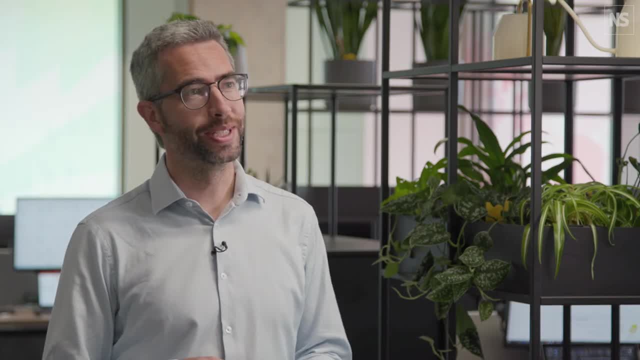 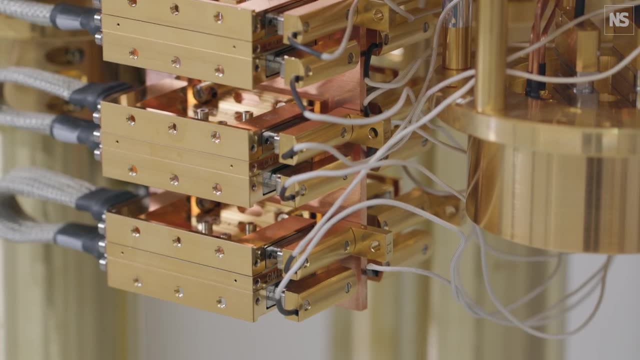 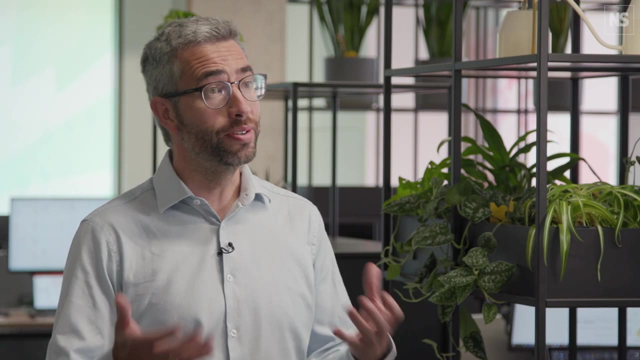 that we know how to build, based on the laws of physics as we know them today. That's possible because they harness the most deep laws of nature- quantum mechanics- in ways that computers today just aren't able to do. Quantum computers can solve problems that are predicted to take longer than the age of the universe. 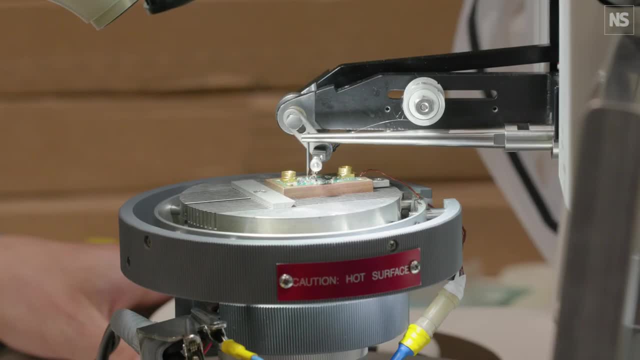 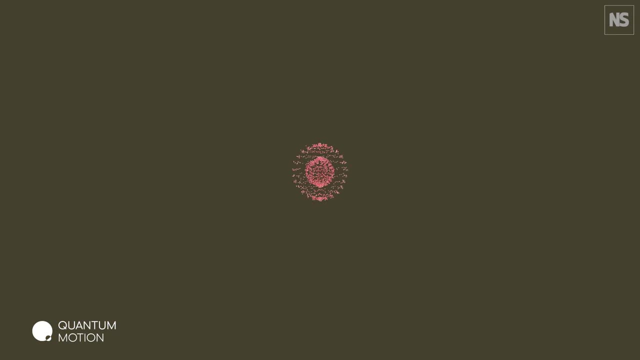 for our bigger supercomputers and solve them in a matter of days, hours or even minutes. Conventional computers encode information in binary bits that can either be zeros or ones. In a quantum computer, the basic unit of memory is a quantum bit or a qubit. Qubits are made using 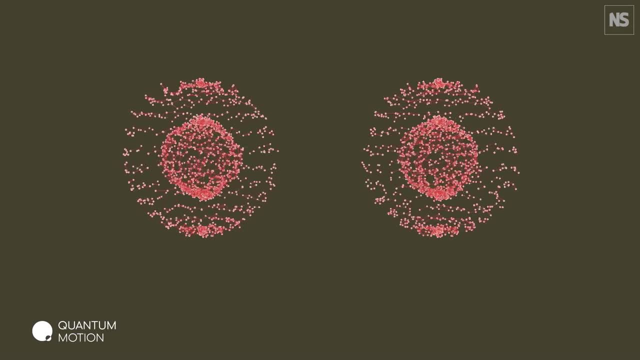 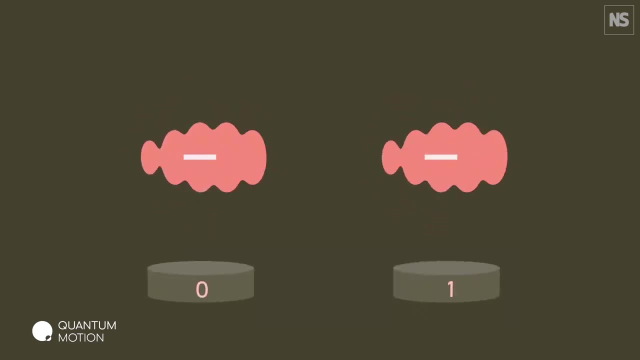 physical systems, such as the spin of an electron or the orientation of a photon. These systems can be in many different arrangements all at once, a property known as quantum superposition. Qubits can also be inextricably linked together using a phenomenon called quantum entanglement. The result is that a series 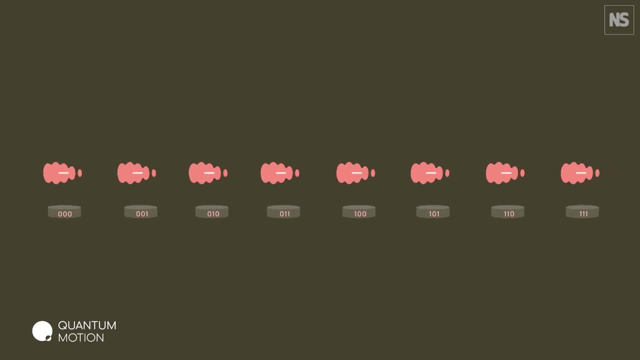 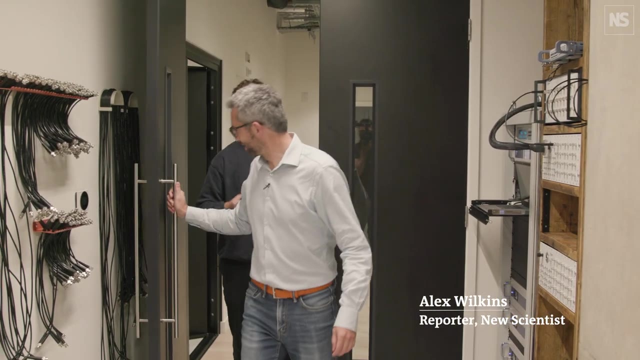 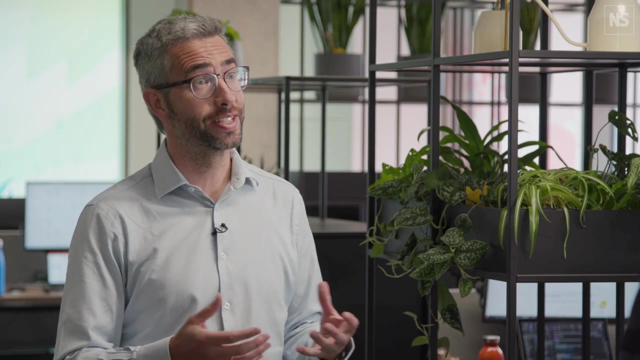 of qubits can represent different things simultaneously. Companies have been working on building quantum computer chips for decades. I'm here in London to visit a quantum startup that's taking a different approach. We're taking one of the most ubiquitous devices in the world today, the silicon transistor. You and I will 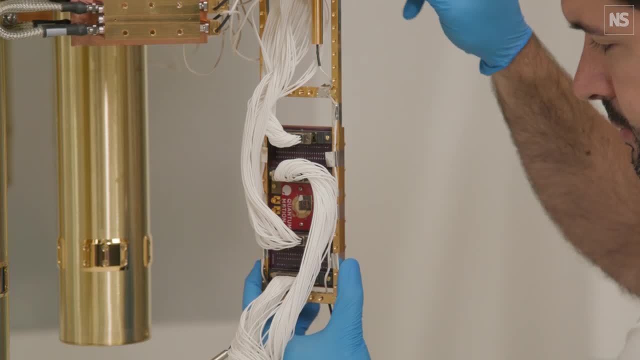 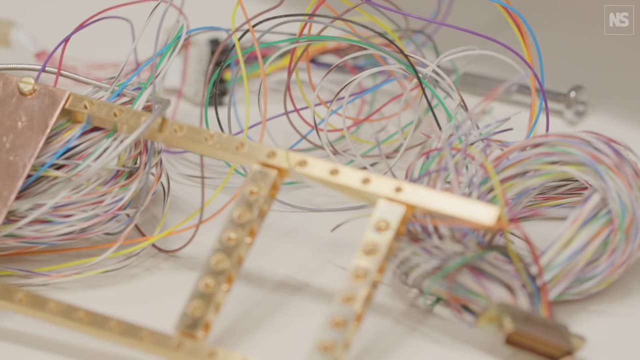 have billions of transistors on our person, in our watches, our computers, our phones- and take that silicon transistor and use that to store a quantum bit or a qubit, And in that way we'll be able to make quantum processors that can scale up and really tackle some of 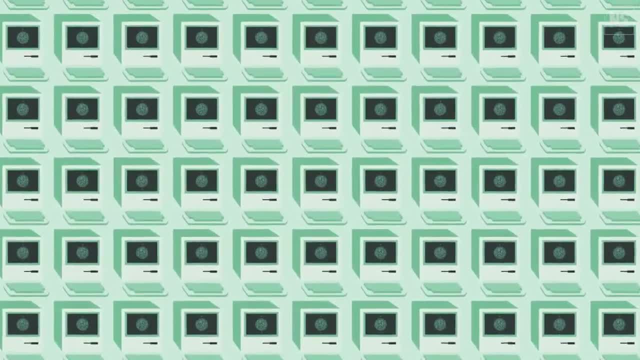 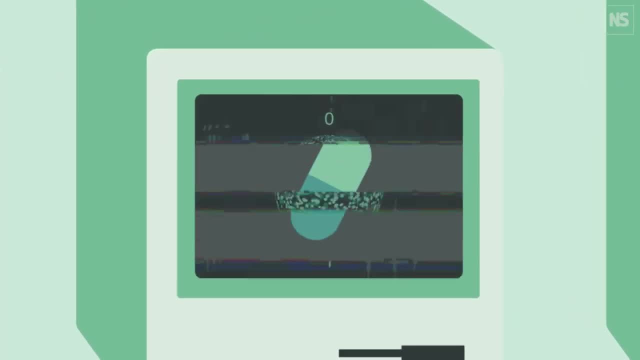 the big problems in computing. Computers today are used for almost everything, but there are some problems that are beyond the capabilities of even our biggest supercomputers, Like producing new chemicals, modeling exotic materials and predicting the weather. All of these processes use the laws of quantum mechanics, which, for today's computers, is 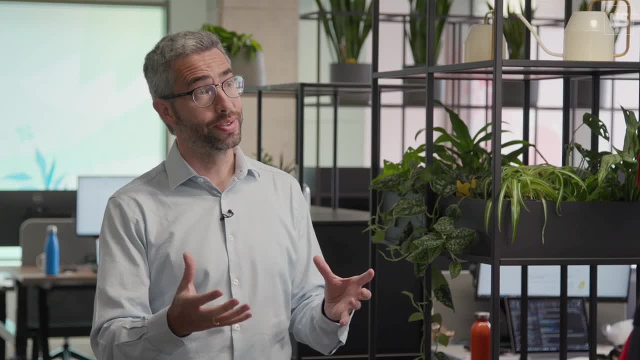 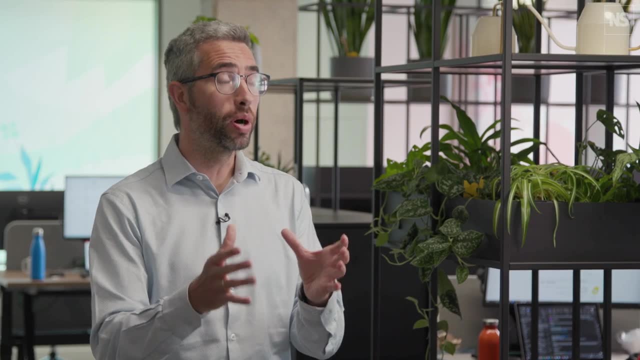 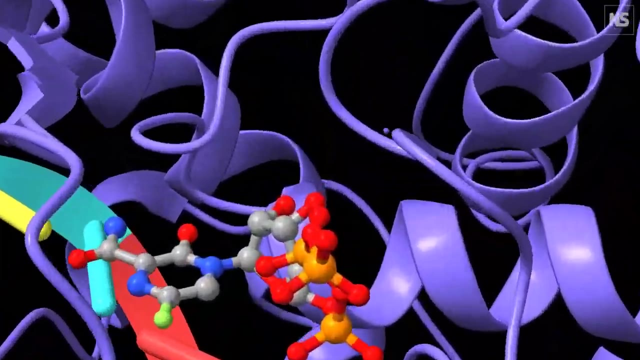 computationally infeasible to incorporate. By using quantum computers that are themselves working on the principles of quantum mechanics, we'll be able to, in the box, in the computer design, new kinds of materials, new chemicals, new drugs, in a way which is much, much faster. 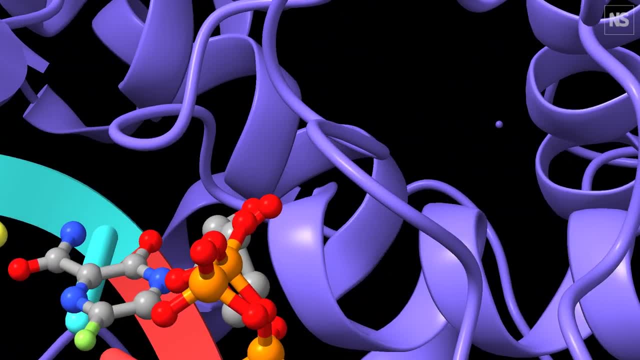 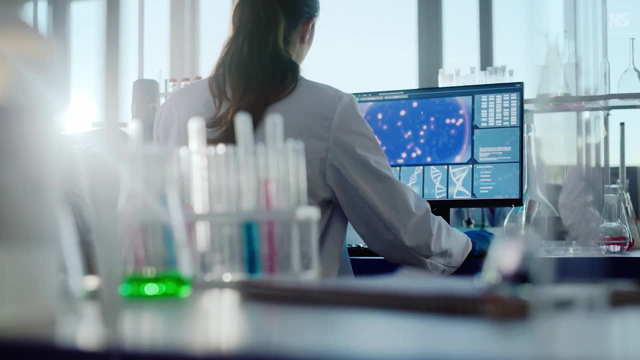 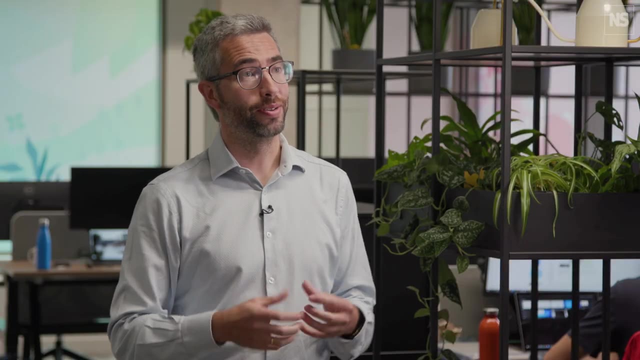 than having to go through laboratory trial and effort, And so we think it could be transformative to tackling climate change through in the future, even to areas like personalized medicine. Building a functioning quantum computer is very challenging, but it's more than just having qubits: You then need to wire them. 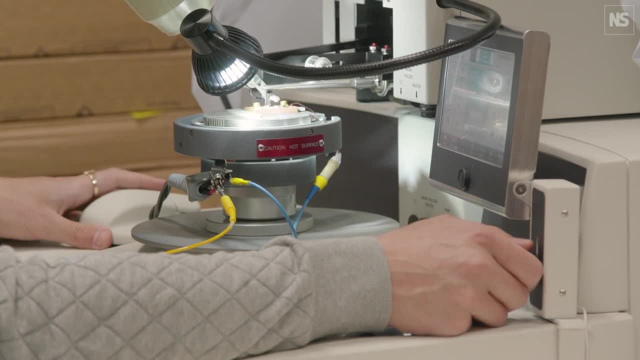 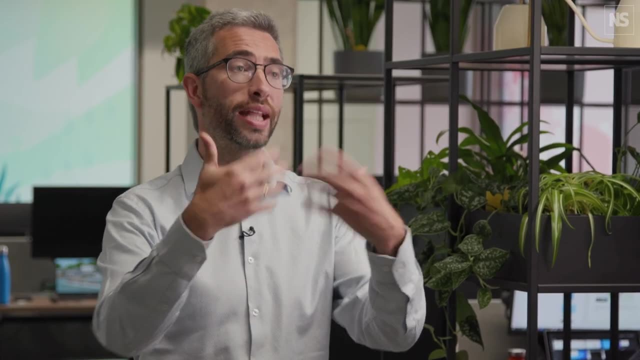 up to be able to run quantum algorithms, And then you need interactions between the different qubits to form that basic unit of computing that allows you to run the process. And in order to keep a quantum computer functioning, you need to keep it cool. 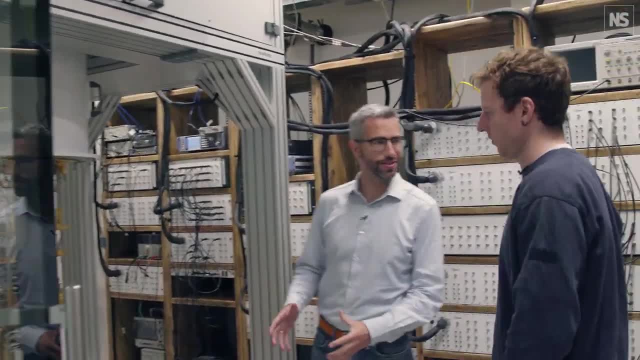 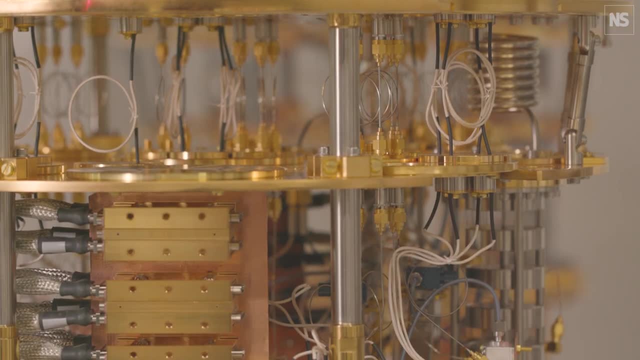 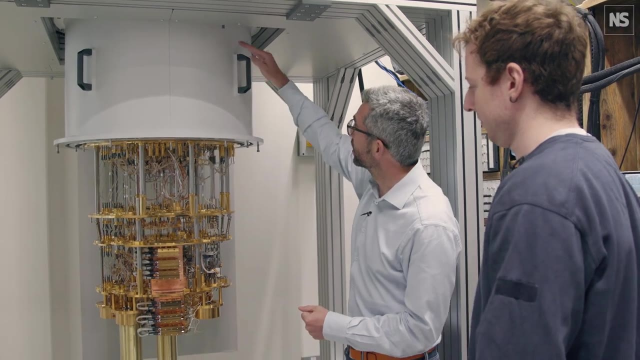 What we've got here is one of our cryostats. It's known as a dilution refrigerator, and we use it to cool down our quantum chips to a hundredth of a degree above absolute zero. This cryostat works in. it has different stages. When it's cold, there's a plate here. 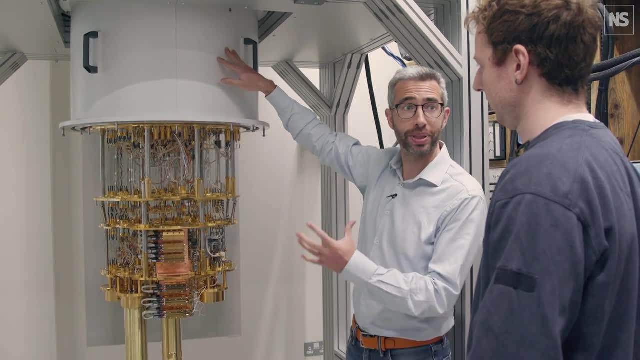 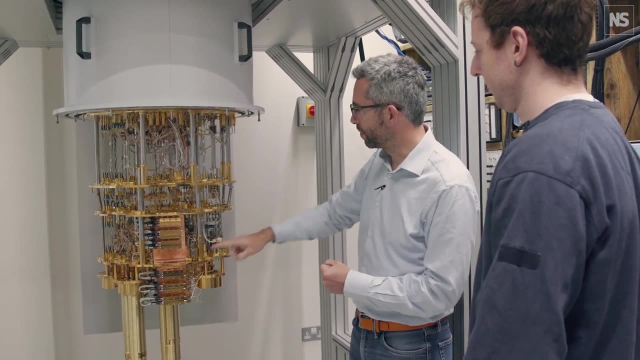 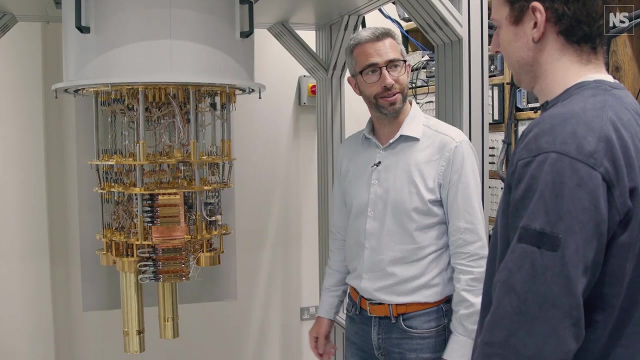 which is a temperature of one of the planets more distant planets in our galaxy. This plate here is about the temperature of deep space, And then this plate here is a hundred times colder than that, about 10 millikelvin, or a hundredth of a degree above absolute zero. 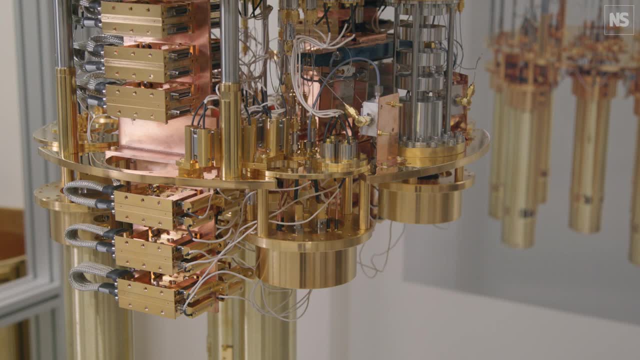 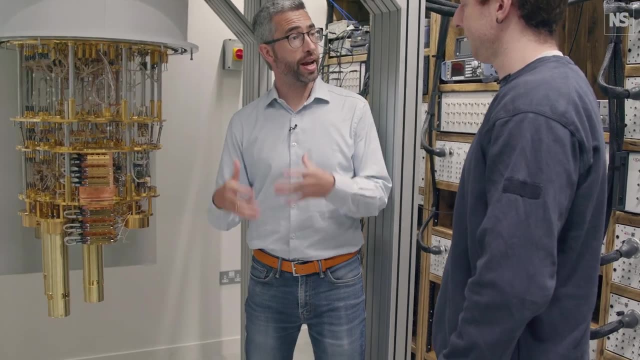 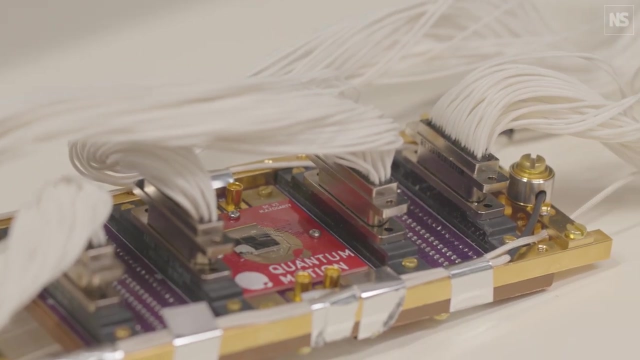 Why does it need to be so cold down here? What's happening in this area that's not happening up there? We want to cool our chips down to very low temperatures to suppress noise and errors and allow these single electrons to be well behaved as qubits in the silicon chips. 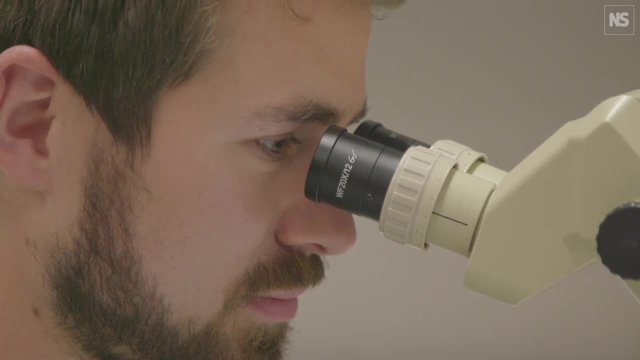 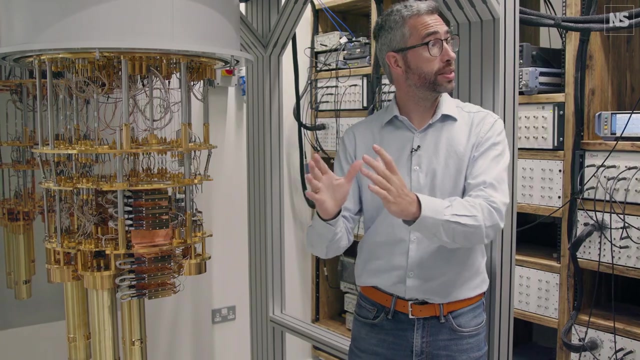 At the moment we're very much in an R&D phase, right, We're developing the technology, So a lot of what you see here wouldn't be required for a standalone operating quantum computer At the moment. we want a lot of flexibility. 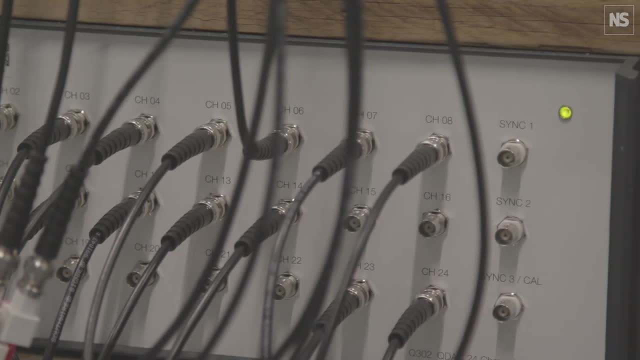 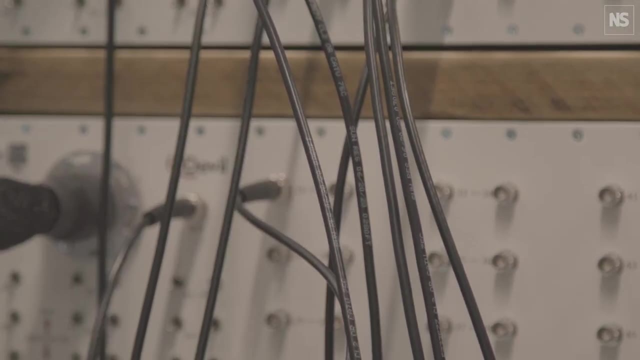 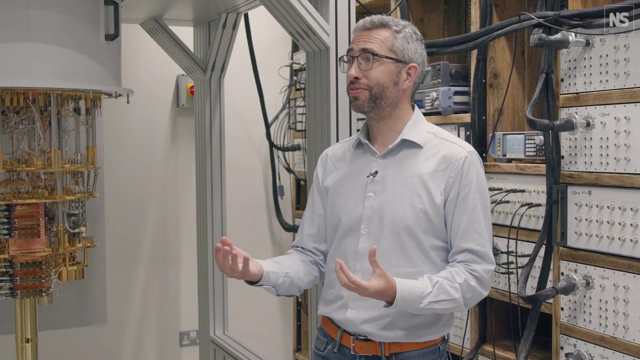 We want to be able to change the types of measurements that we're probing our chip with, But pretty much everything that you can see in these racks could be miniaturized to a very small controller. But the great thing is that now, with cloud computing, the user from a smartphone can access.